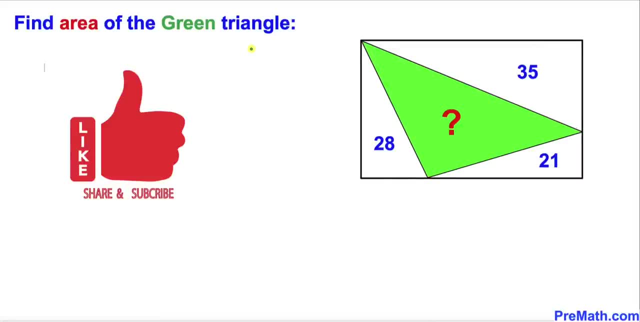 Please don't forget to give a thumbs up and subscribe. So let's go ahead and get started with the solution, and here's our very first step. Let's go ahead and label these side lengths of this rectangle. Let me go ahead and label this side length as x and this side length as y. 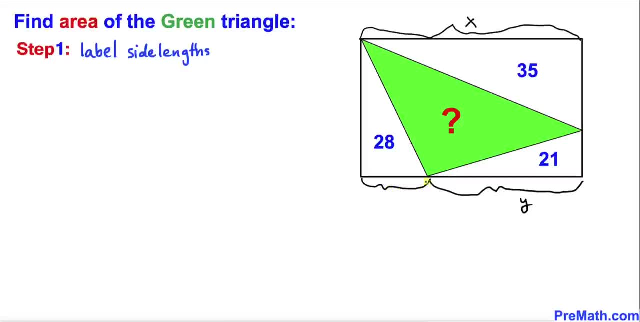 Then this side length is going to be simply x minus y. and now let's focus on this shaded triangle. Now let's recall the area of a triangle formula. and here's our area of a triangle formula. Area equals to a half time base times height. Now 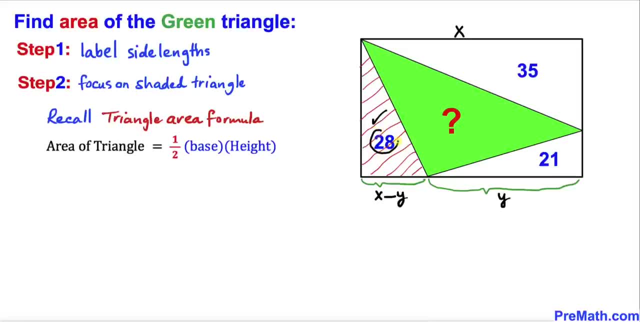 in this shaded triangle. our area is 28 and our this base is x minus y. Then our height has got to be 56 degrees divided by x minus y. Now you might be wondering: how did I get this 56 divided by x minus y? 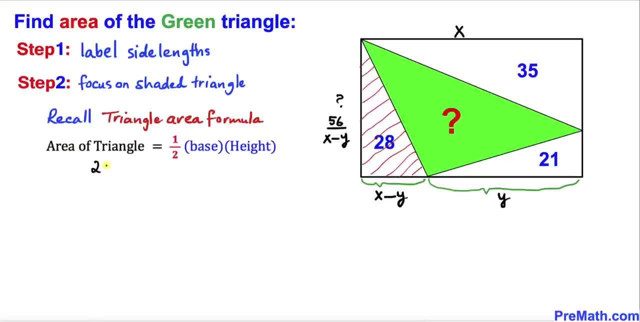 Let's go ahead and plug it in. Our area of this shaded triangle is 28, equals to a half, and our base is x minus y and our height is 56 divided by x minus y. and here x minus y and x minus y is gone, and the right hand side, 56 divided by 2, is 28 and the left hand side is 28.. 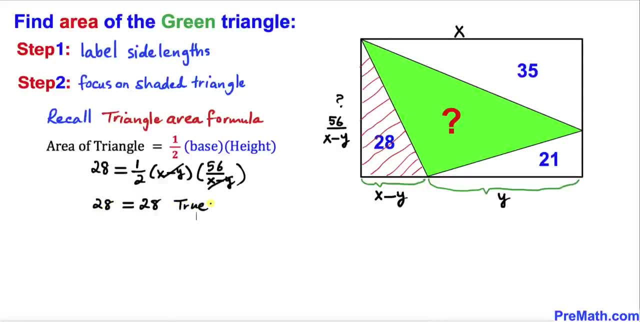 So this is indeed a true statement. and now let's focus on this, another shaded triangle. Our this side length is x, which is our base, and we know the area is 35, so this side has got to be 70 divided by x. And now let's focus on this triangle. Our area is 21 for this shaded triangle and this side length. 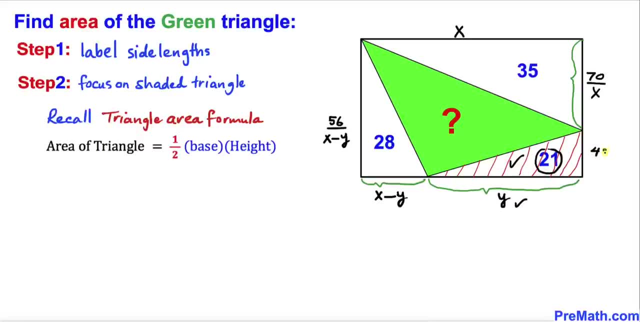 is y, then this side length has got to be 42 divided by y. And here's our next step. Let's focus on this rectangle. as you can see over here, These two sides, these opposite sides, are equal in length. are going to write down this: plus this equals to this: let me go ahead, write down this one: 70. 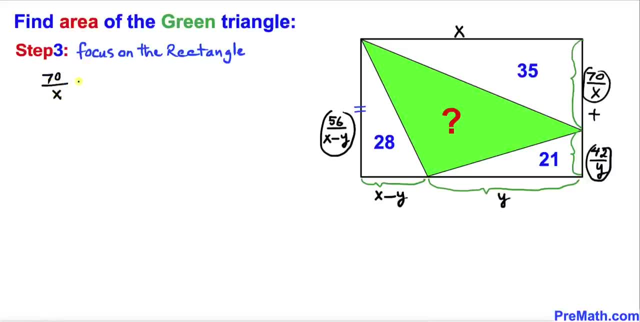 divided by x plus 42 divided by y, equal to 56 divided by x minus y. and now we can see, all these numerator numbers are divisible by 14. so therefore, I am going to multiply these both sides by 1 over 14 and I am going to distribute that one and that is going to give us 5 divided by x plus 3. 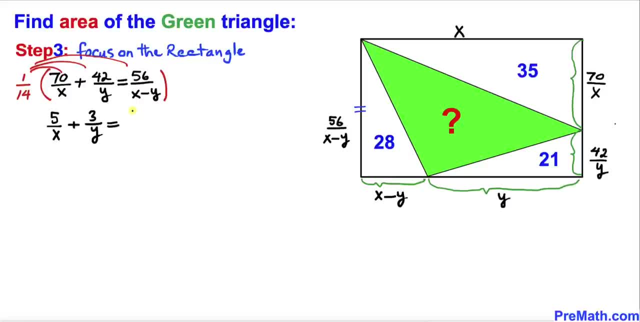 divided by y equals to 4 divided by x minus y. now let's go ahead and add these two fractions on the left hand side by using the crisscross method, so that could be written as 3 x plus 5 y on the top, divided by x times y. 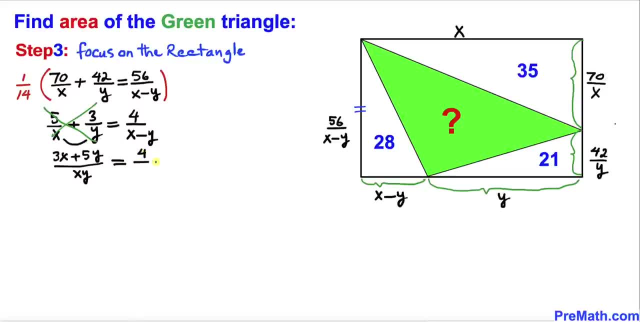 and the right hand side is going to stay same: 4 divided by x minus y. and now let's go ahead and cross multiply so we can y. and now let's go ahead and cross multiply, so we can y. and now let's go ahead and cross multiply so we can. 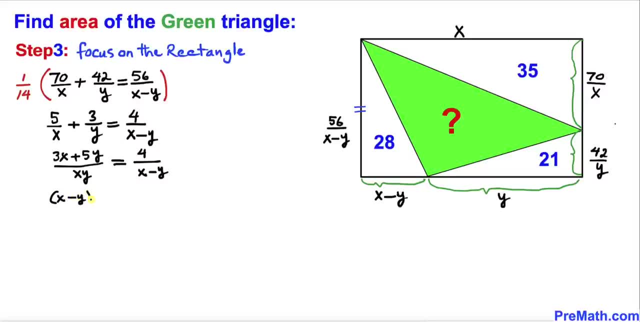 write this one as x minus y times 3x plus 5y equals to: on the right hand side is going to be 4 times x- y. and now let's go ahead and do the double distribution, or sometimes we call it rainbow method. so that is going to give us 3x square plus 5xy minus 3xy minus 5y square, equal to: 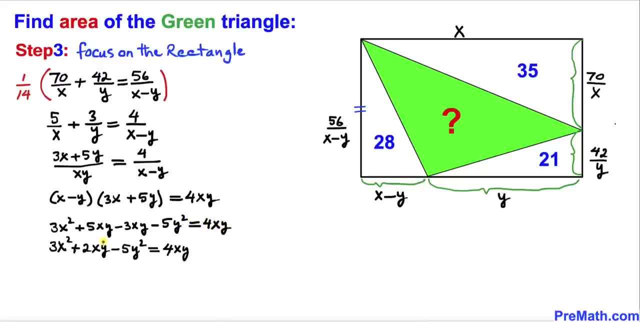 4 times x- y. now, in this next step, 5xy minus 3xy is going to give us 2xy, and the right hand side is going to stay the same. so let's go ahead and do the double distribution, or sometimes we call it. 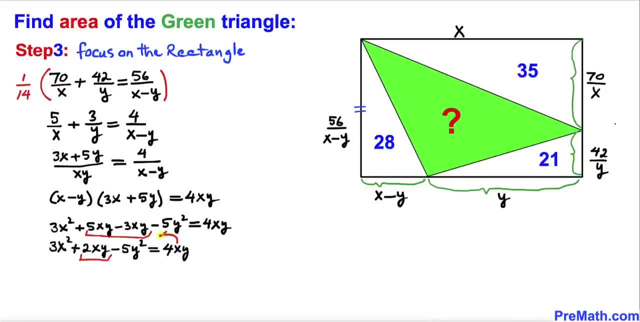 4xy. now let's move this 4xy on the left hand side as well. and here I moved this one negative 4xy on the left hand side. let's go ahead and combine these two like terms equal to zero, and now we can see that we got this quadratic equation and we're going to solve it by grouping and. 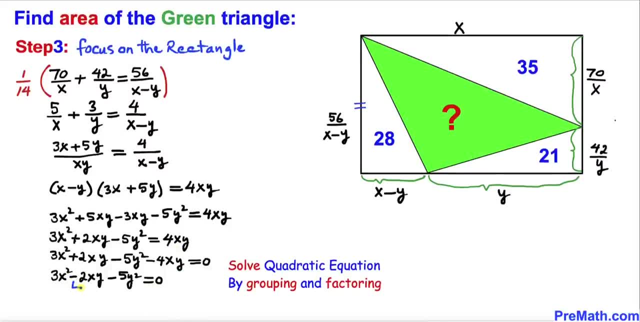 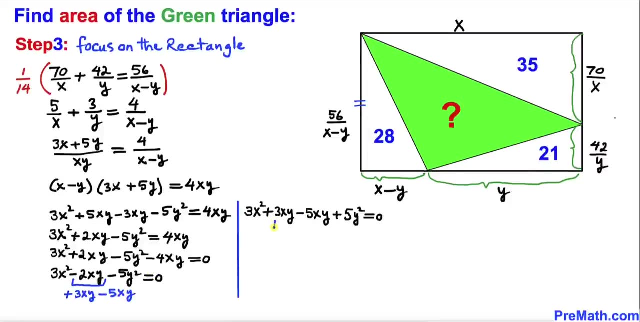 factoring. so therefore we are going to tweak this negative 2xy, we can write this one and we're going to do the double distribution, or sometimes we call it rainbow method. so that is positive 3xy minus 5xy, and here I have replaced this negative 2xy by this positive 3xy minus 5xy. 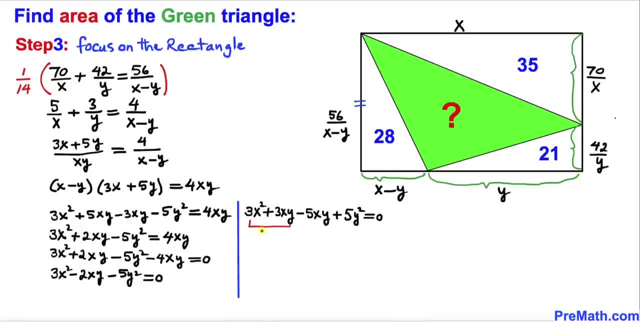 and now we can see: between first these two terms, 3x, is in common, and between these last two terms, negative 5y is in common. so let's go ahead and factor this one, 3x, out of the negative 2xy. and now we can factor out the negative 2xy in common if we do these twoせて both by multiplying two. 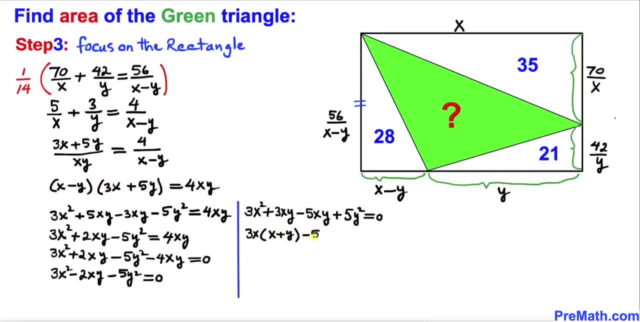 empty j总 out here. we are just going to turn the Oscars in one place and every point takes one point minus the other in templ preciso. if we do this, новast, we are going to be tempted, in the third place, to multiply these. Germany, we are not yetkal. 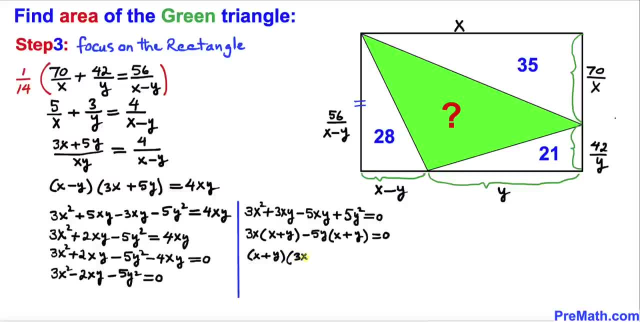 and now we can divide into two each other so that we will roughly be able to see that, the meaning of the extremes, and so that will be known to people. our solution is going to be that there is a combination of two important terms. so these are the two things we are going. 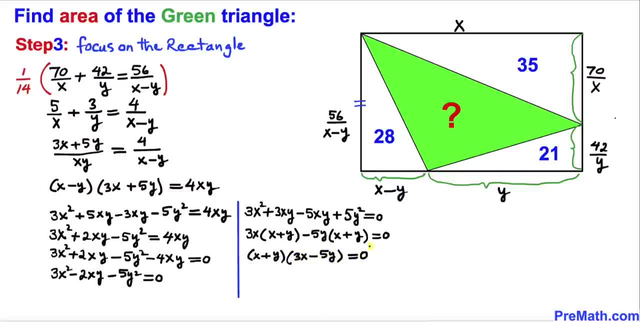 to arm and there are the week. so we are going to change the zero down curve to two. these also we will be able to analyze with the denominator, such that if we wanted to now say that equal to 0, and now let's go ahead and separate them, I can put x plus y equal to 0, and on this, 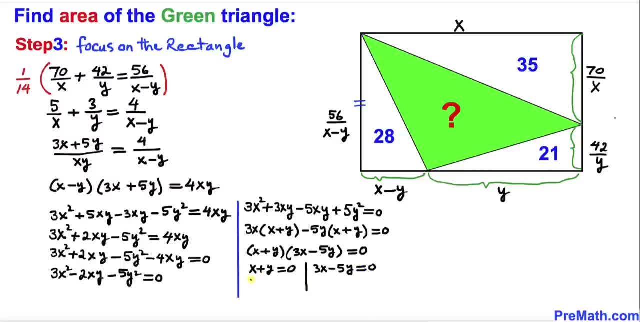 side equal to 0. so that is going to give us x equal to negative y, and now we can see that this is not conducible. so therefore we are going to reject this one. Now let's focus this part of the equation. so this could be written as: 3x equal to 5y and now divide both sides by 5. so that means: 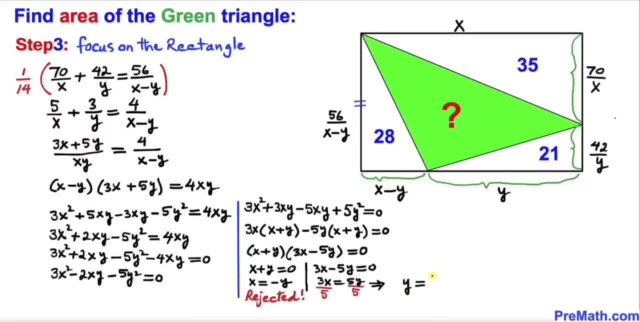 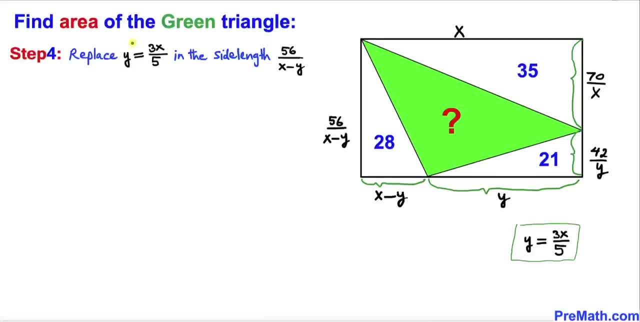 our y value turns out to be simply 3x divided by 5. and here's our next step. Let's go ahead and replace this y equal to 3x divided by 5 value in this 56 divided by 0.. x minus y. and now we are going to replace this y by this 3x divided by 5, so this could be written: 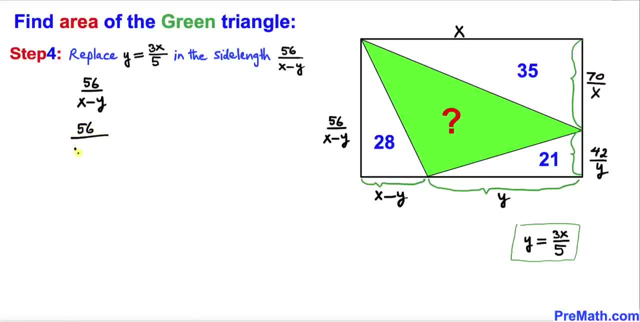 as a 56 divided by x minus 3x divided by 5. and here i have copied down this whole denominator over here, and if we simplify, that is going to give us 2x divided by 5. so therefore we can write this thing as 56 divided by 2x divided by 5. and now this 2x divided by 5, we flipped it over and 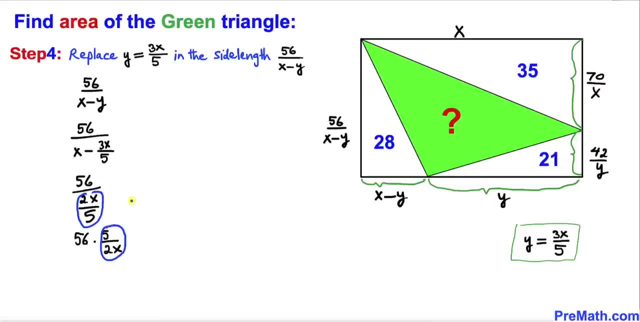 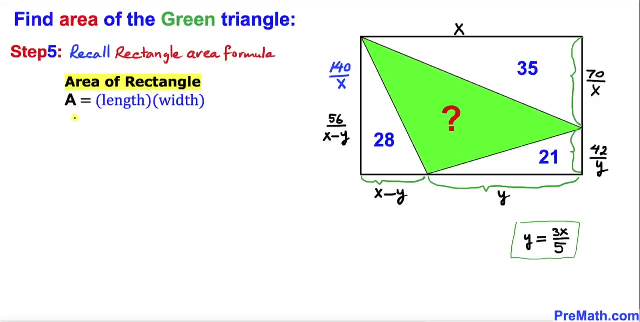 multiplied by 5 divided by 2x, and that turns out to be 140 divided by x. so therefore, i'm going to replace this one by 140 divided by x. and here's our next step. let's recall the rectangle area formula, and here's the area of a rectangle formula. area equals to length. 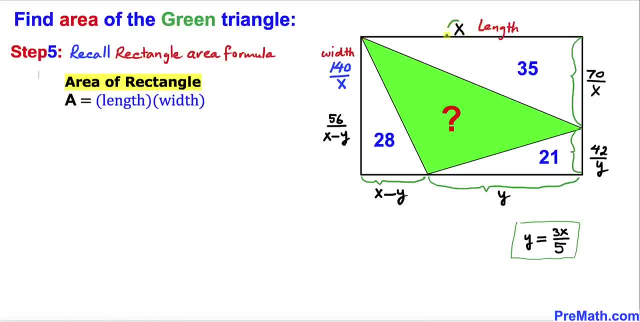 times width. and here, in our case, our length is x of this rectangle and the width is 140 divided by x. so let's go ahead and plug it in. so area of this rectangle is 140 divided by x. so let's go ahead and plug it in. so area of this rectangle is 140. 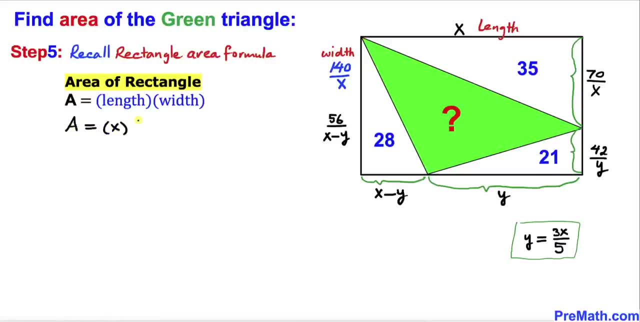 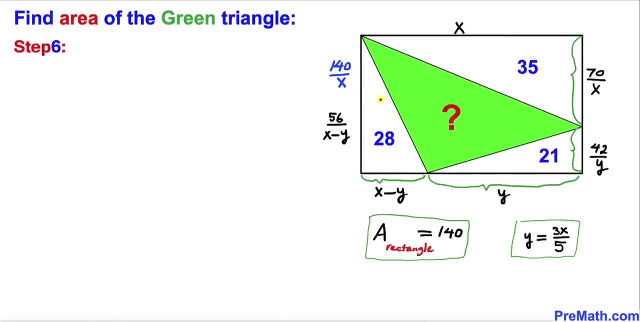 and here still, we are going to see that the angleется, the x value of this triangle point looks like the. so area of this triangle is going to be: length is x times trav leven, and our final step here is the area of this triangle comes to be a dan is this area and it's area of this triangle and here's our final step. let me call this area of this triangle as a1 area of this triangle appeared to area of this triangle, a3 and nine two and the area of this triangle.